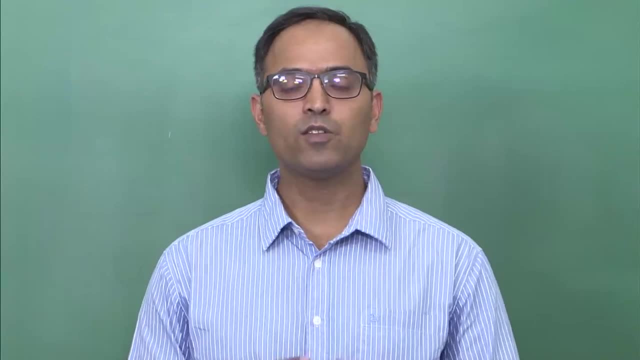 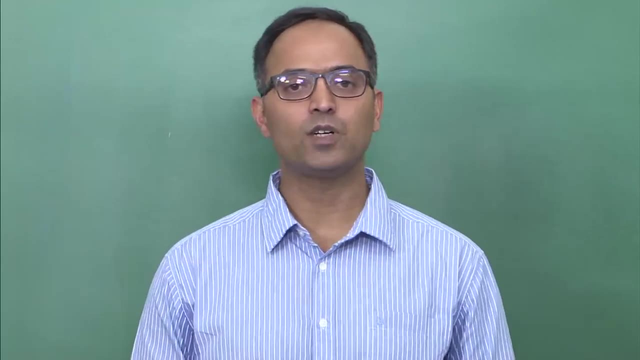 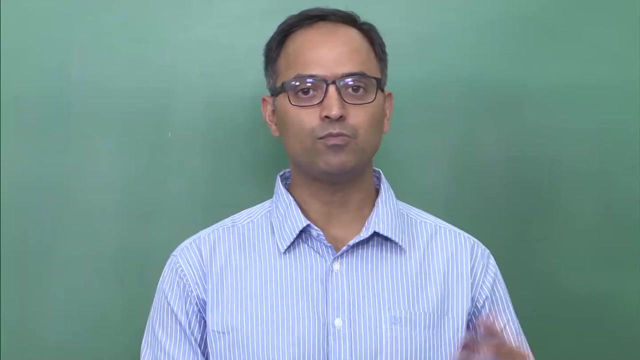 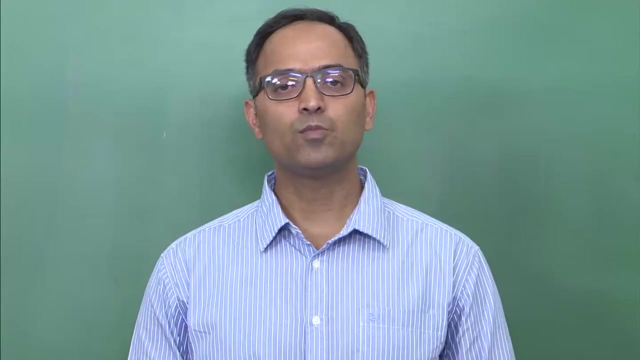 know the property of the materials. The property of the materials in this case, which depends on temperature and pressure. you have to choose a specific set of properties. properties such as odorless or other property which are relevant for potable water, for example, is not relevant for thermodynamics. In thermodynamics, the properties which are related to energy. 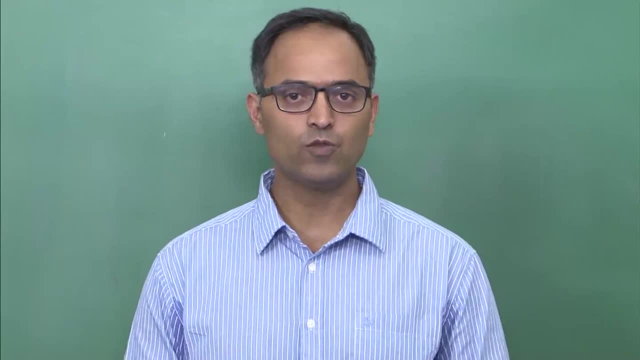 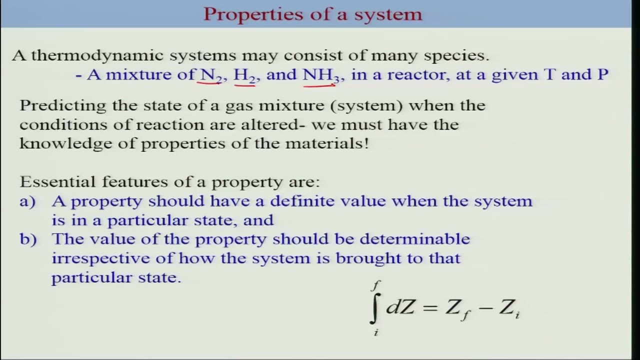 and its transformation are only useful in the analysis. So right. so the essential features of a property would be that it should have a definite value when the system is in a particular state. Again, as I said, properties such as odorless or testless are not useful in the 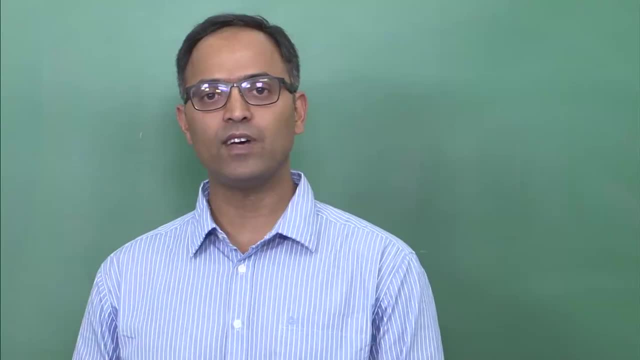 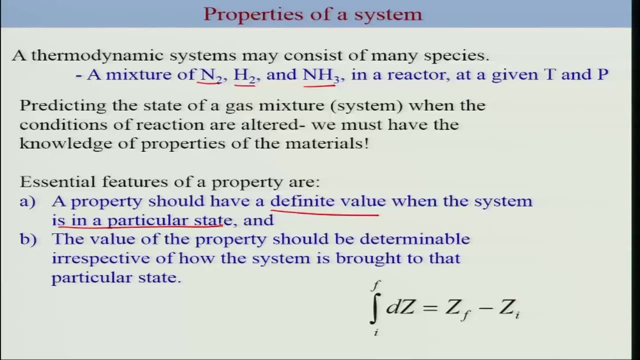 thermodynamics analysis, you have to choose properties which has a certain value which is related to the energy or change in energy. So a property should have a definite value. when a system, which is a specific state, and the value of the property should be determined irrespective of how that particular state is changed, So the property should have a 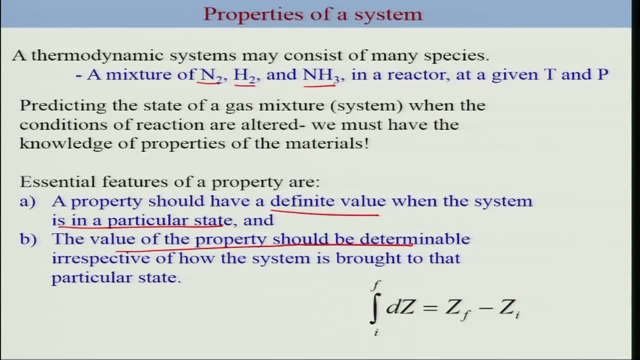 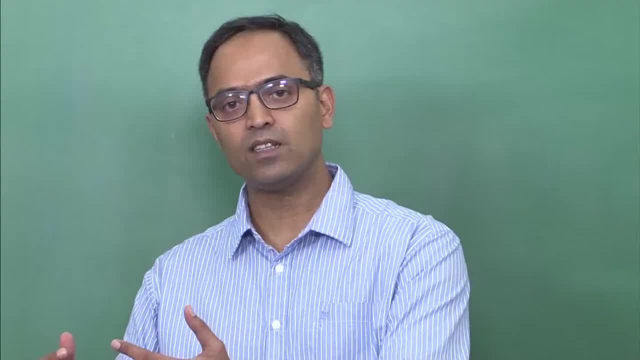 definite value when a system reaches a specific state and the value of the property should be determined irrespective of how that particular state was achieved or was brought to that particular state. So it does not matter how the state was achieved. the property should depend on the final value. So the change in the property from one state to another. 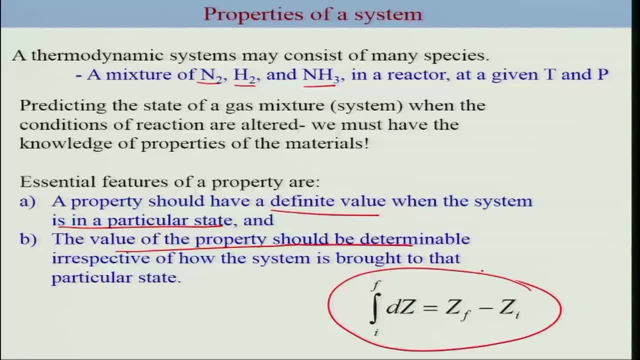 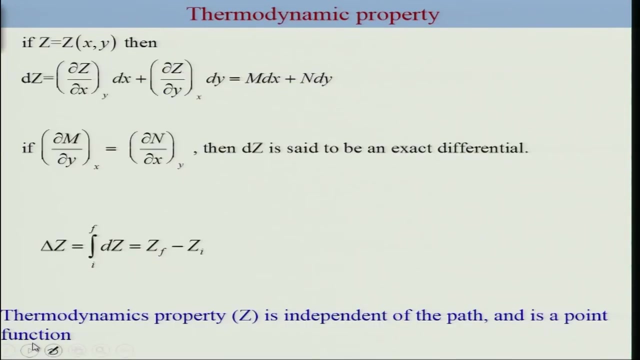 state can be clearly written in this expression: where Z is a specific property and it changes, a change in the Z value from some initial state to the final state is given by the difference between these two values. Now let us little bit look at the mathematics. So if you say Z depends on a two variable, 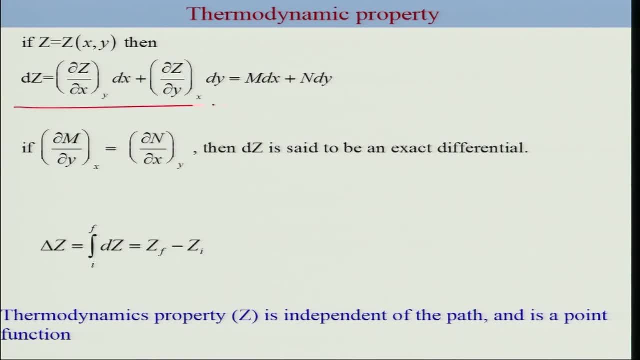 X and Y. you can write the differential of Z in the following form: where the partial differential of Z with respect to X is given by M and this is M, and mathematics tells us that if this condition holds, then the DZ is said to be exact differential. 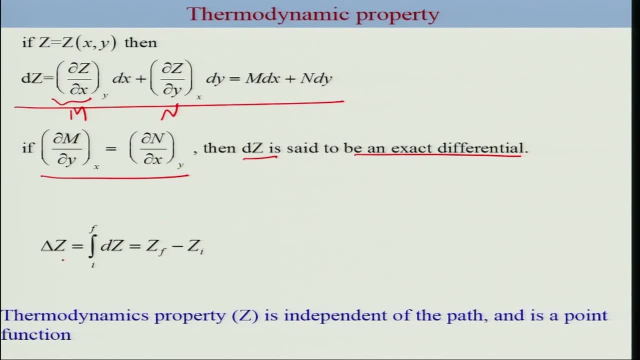 Now, in such condition you can integrate this in this form. that means you can write del Z as a integral of DZ from I to F, and this would be given as the difference between Z of final and the initial values, And therefore thermodynamics property Z is an independent. 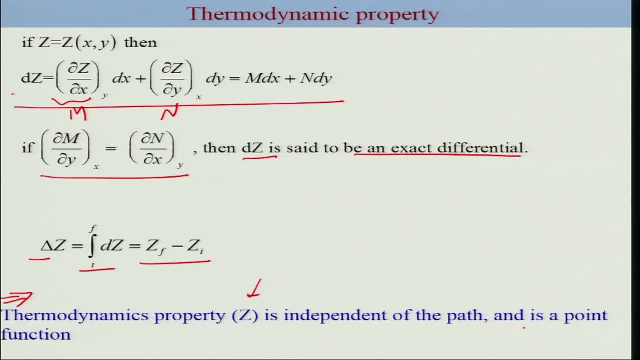 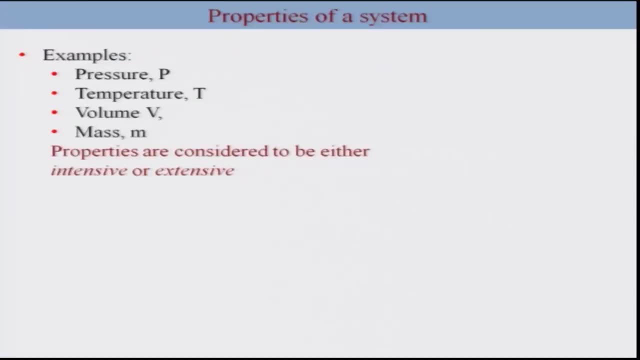 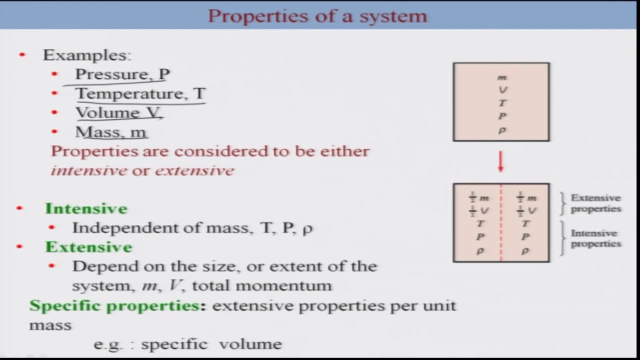 of the path because of being exact, differential and is a point function. So this is a definition of the point function. So let us look at common properties of a system. The examples are pressure, temperature, volume and mass. The properties can be extensive or intensive. So just take an example, Let us consider: 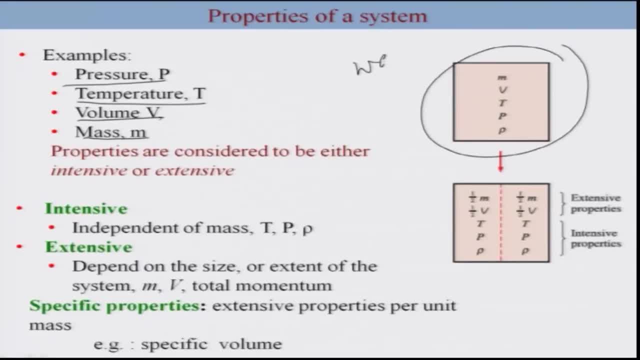 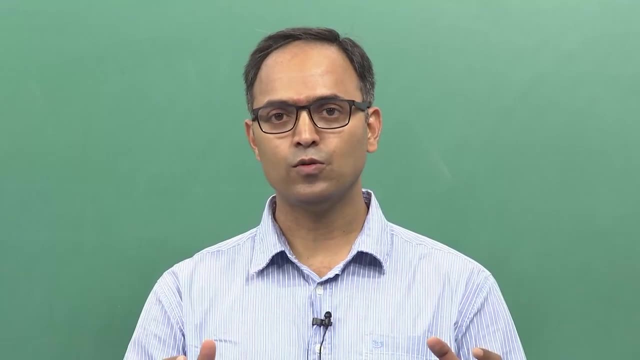 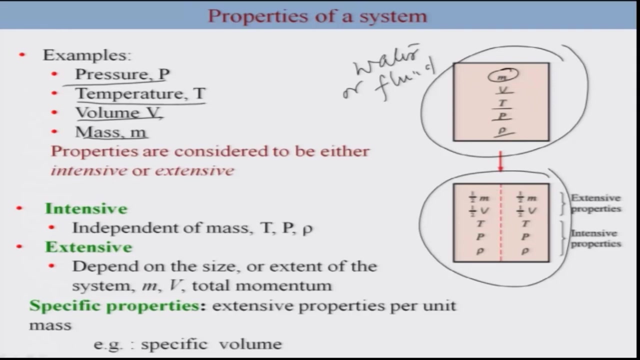 a system. This system can be simply water or any fluid having a mass, M, volume, v, temperature, T, pressure, p, rho. Now you divide this particular system into two parts, and that you can do in this form, where you have divided into two, part one and part two. Now the mass certainly gets. 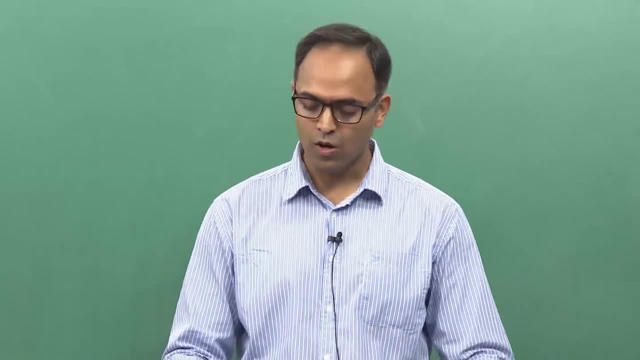 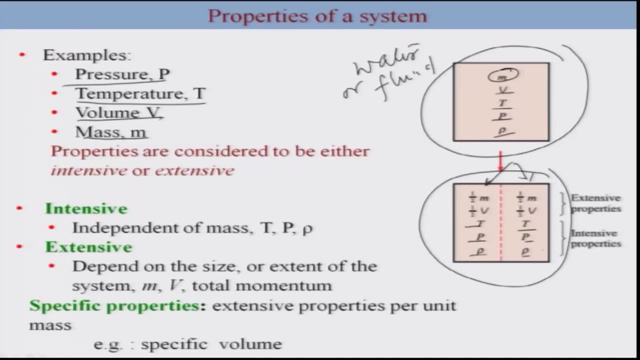 divided by two, volume certainly gets also divided by two. On the other hand, temperature of both the parts should remain same, the pressure should remain same, and as well as the density. That is what we can understand from our daily experience by taking water in a glass and dividing into two parts. So certainly certain properties are affected. 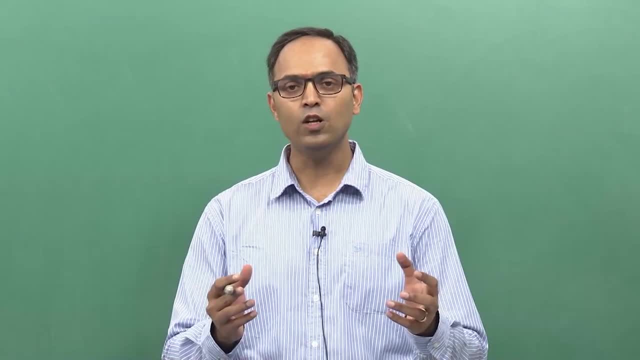 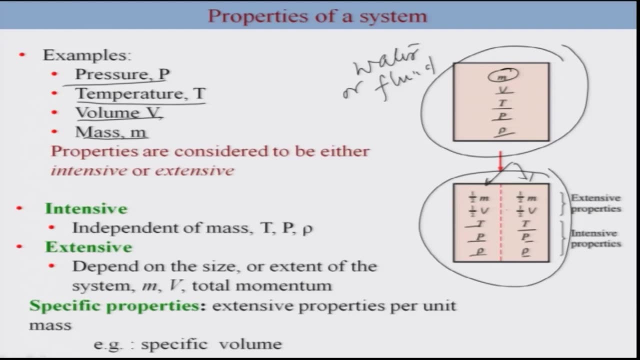 by this aspect of, let us say, division of the volume, which means it depends on the volume or the mass. On the other hand, the other properties do not, such as temperature, pressure and density. So that becomes the basis for categorizing properties into intensive and extensive. So 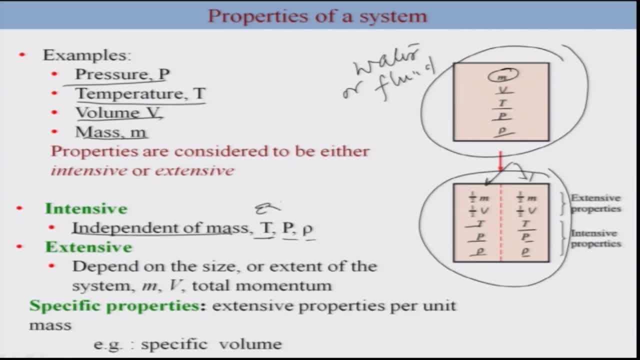 intensive properties are independent of mass. Examples are temperature, pressure and density. And extensive properties are which depends on size or extent of the system: Mass, volume, total momentum. these are the extensive properties. Now there are other properties, which are called specific properties, which are extensive properties per unit mass, such as specific volume, which 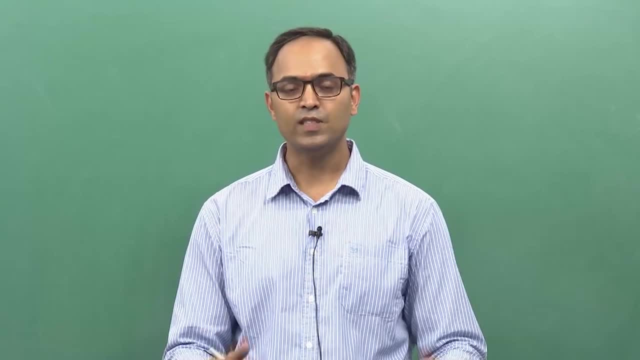 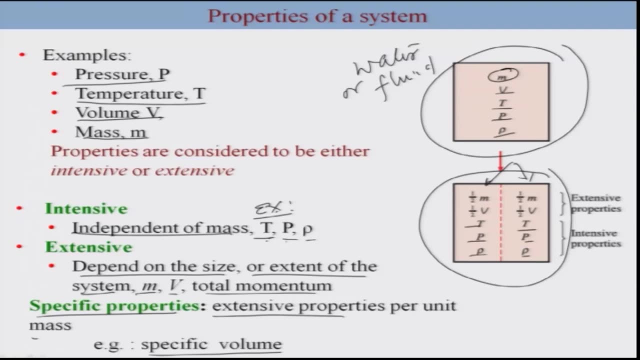 is basically volume divided by mass, And specific volume becomes the intensive property. So typically the intensive properties are the volume divided by the mass, And the volume of the mass is a mass. that is, the specific amount of mass, and mass is a mass that is: 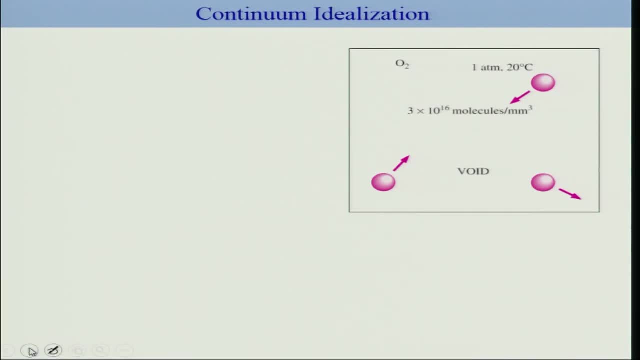 the specific kind of mass And the specific properties are intensive property such as specific volume. Now, in a typical matter, well, the matter of, we know contains of many different atoms, but for us we do not see these molecules or atoms around. For us it looks like a homogeneous. 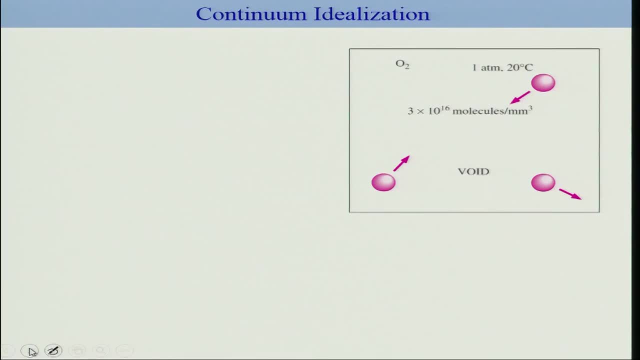 And this is what we are going to use as an approximation. We are going to use the system, these two atoms here. in this case this will be of the order of 10 to power minus 9 meter, okay. And for example, this is oxygen in certain volume at a one term atmosphere, at 20 degree. 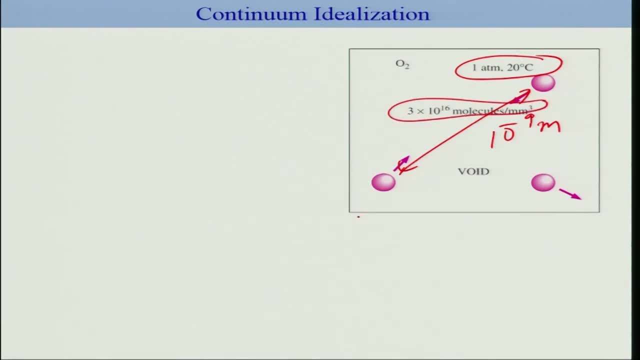 Celsius and there are these many molecules in the system. So if you look at this distance and divide by this distance, the order of L by L is going to be extremely small and in such case this matter will look like continuous, and this is what the approximation we are going to use. 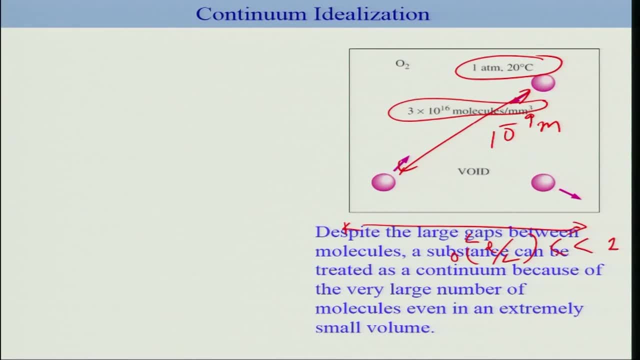 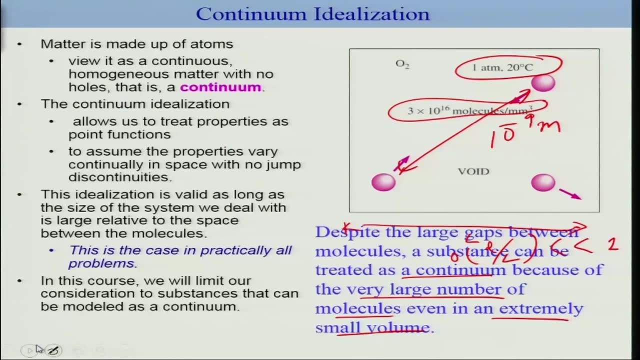 So, despite the large gaps between molecules, a substance can be treated as a continuum because of very large number of molecules, even in extremely small volume. Now this allows us to do consider that the properties are also continuous, So it allows us that property vary continually. 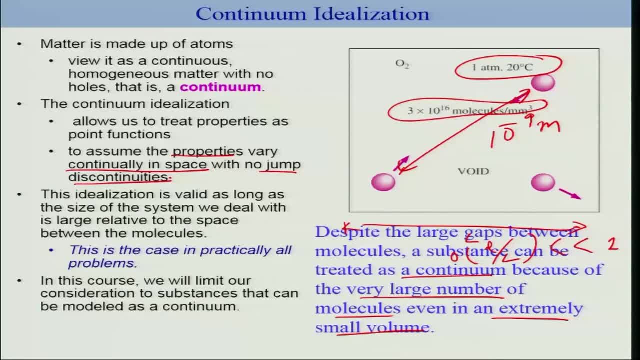 in space with no jump discontinuity and considering the system which we are going to look at, because of the size of the atoms, which are extremely small, this would be the practical case for all our problems. okay, So we are not going to take sand particles or grain. 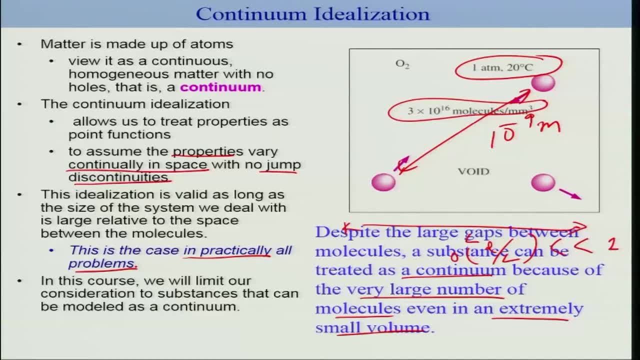 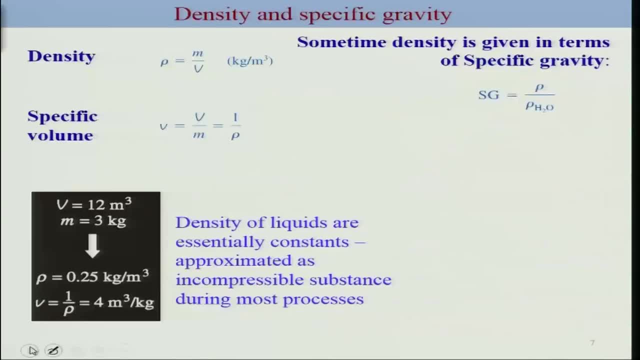 or asteroid, which are extremely large or large in size. So in this course we will be limiting our consideration to substances that can be modeled as a continuum. We will consider this kind of definition. So definition of density is very well known: mass by volume. Specific volume is going to be volume by mass or 1 by inverse. 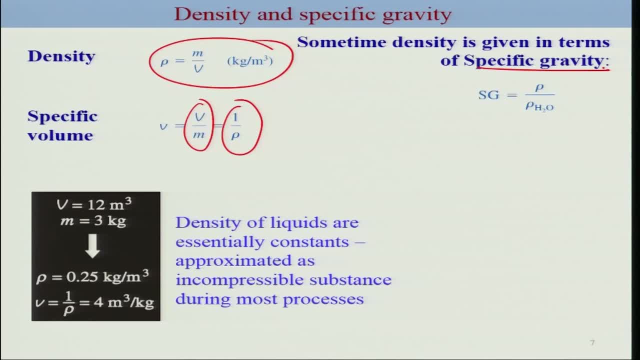 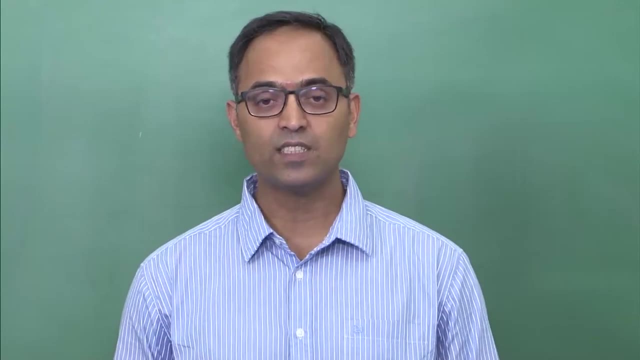 of density. Now you have this specific gravity also, which is the ratio of the density of the substance with the density of the water. Now this density of the water will be considering at 4 degree Celsius, where the density of the water is maximum. Now you can look at the 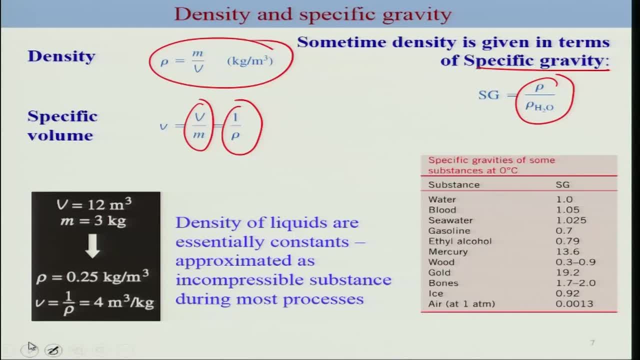 specific gravity for various different substances. Some are greater than 1,, some are less than 1.. Those which- those having specific gravity less than 1- will float on top of the water's layer. okay, Now, density of the liquid- are typically constant and we will be considering to be constant, So that is why they are part. 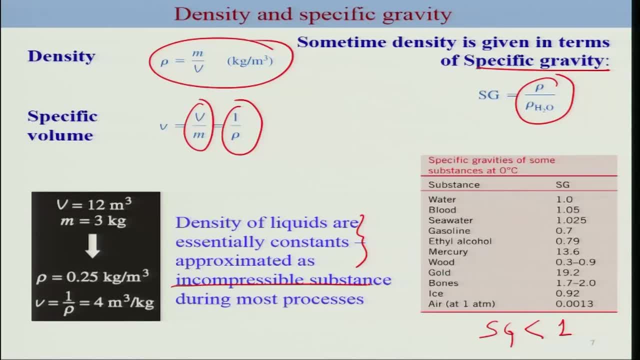 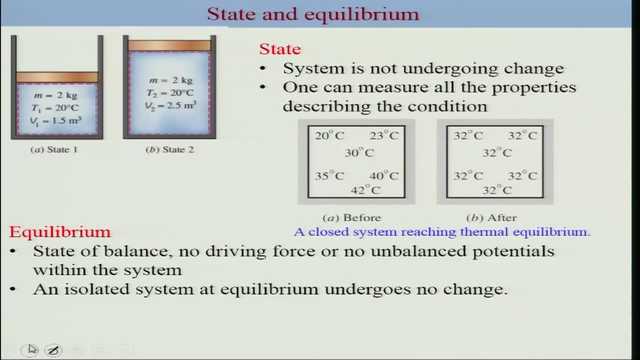 of called incompressible substances, Though they are slight change if you increase the pressure substantially, but otherwise we will be considering a constant density in this particular course. Defined few things. what is the definition of state in thermodynamics? So let us consider. 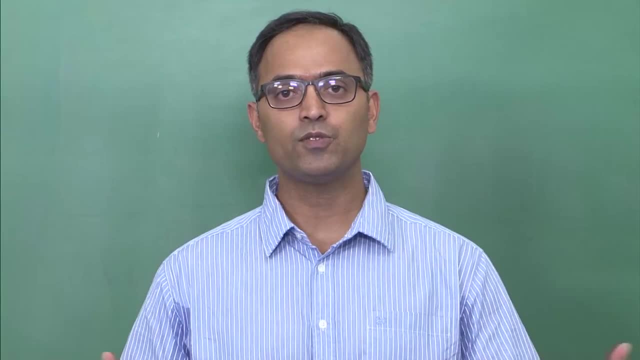 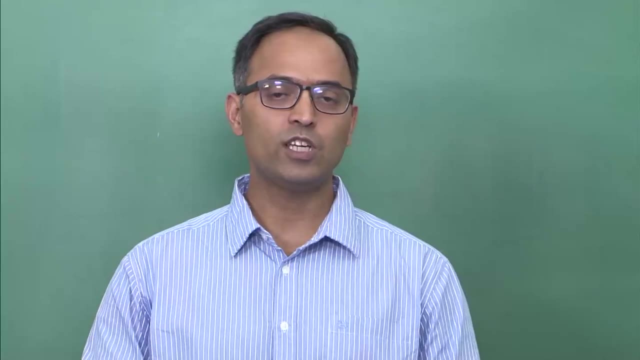 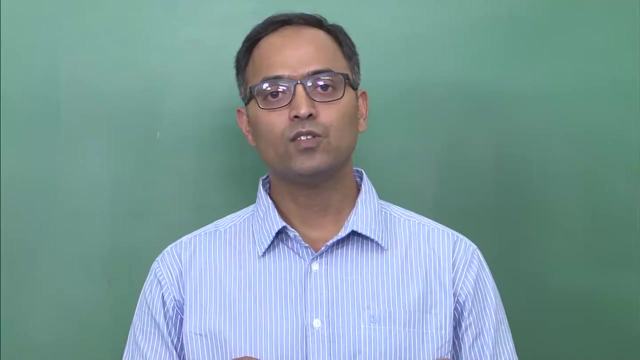 a system which finally stops changing at all, you know. So it undergoes a change and then reaches an a point where no changes in the properties are seen. In such case one can measure the properties, all kind of properties. So a specific state means a specific values. 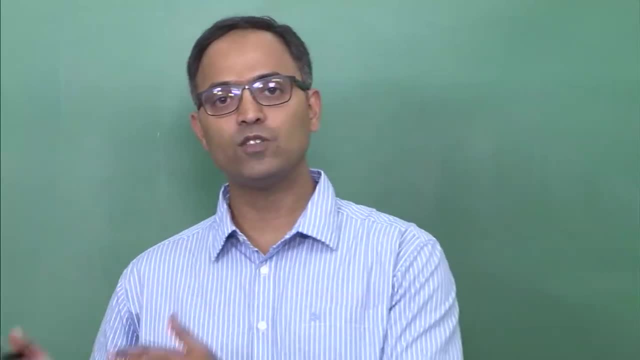 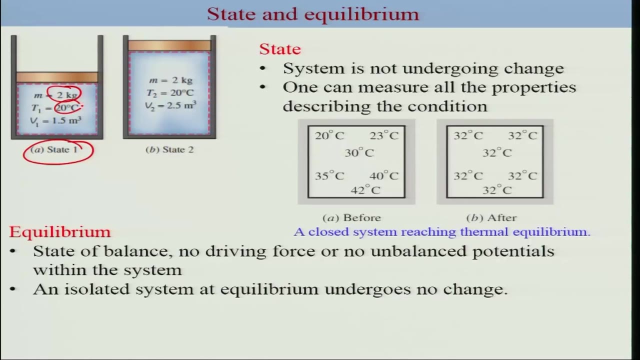 of the properties. So you fix the values of the property. you achieve a specific value. So you fix the values of the property. you achieve a specific, particular state. and this is an example. You have a state 1 with a mass 2 kg, 20 degree. 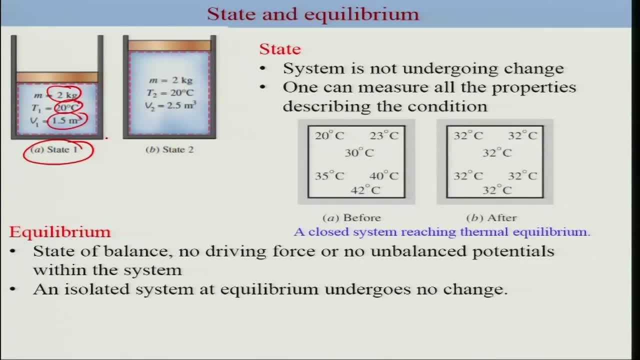 Celsius and 1.5 meter cube. You change the volume to 2.5,. you change the state. You are changing just one property of the state and you are changing the state of the system. So that is how we are going to define the state: having a fixed set of properties. The 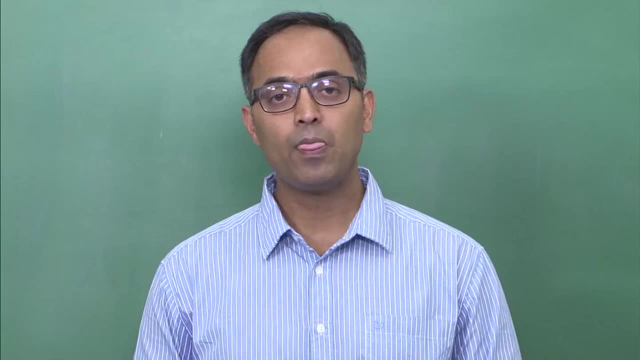 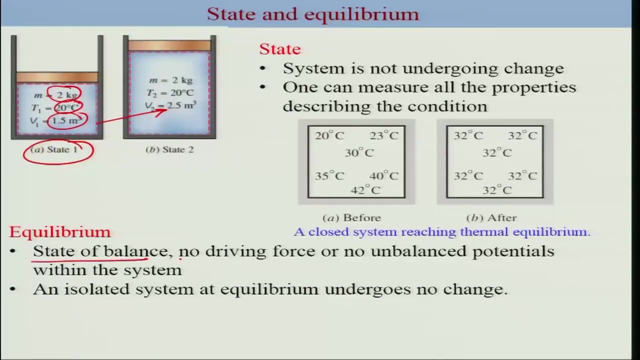 other aspect of thermodynamics we are going to deal with is equilibrium. There are various different kind of equilibrium. So let us look at the equilibrium. So let us look at what is definition of equilibrium. So equilibrium is a state of balance. There is no driving. 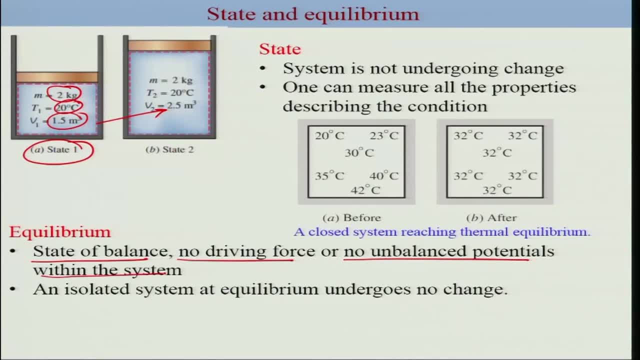 force or unbalanced potential within the system. So let us take a case where you have variable temperatures within the system And, after isolating this closed system, it reaches a continuous or constant value of the temperature throughout the system. So a closed system. 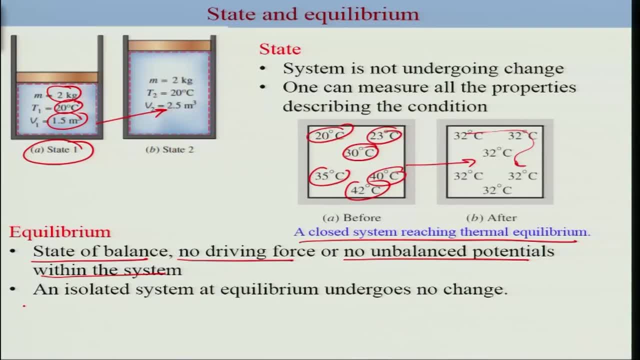 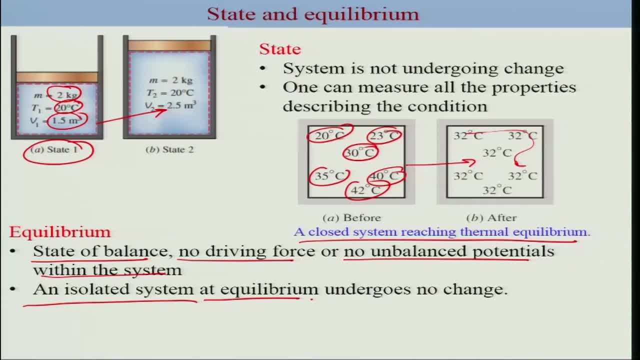 a system and isolate it at equilibrium, there will be no further change. So after this particular system, if you isolate it, there is going to be no change. So even if it is a closed system, let us say, if I do not isolate it and let it equilibrate to a specific temperature. 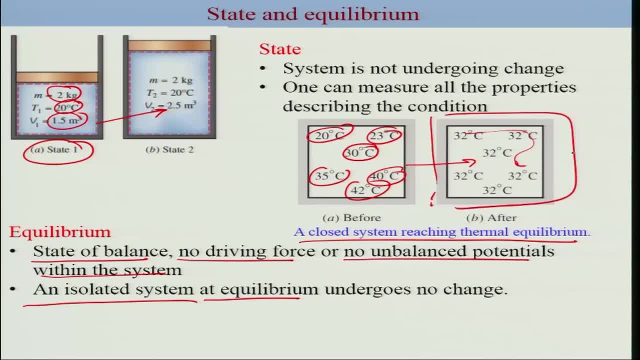 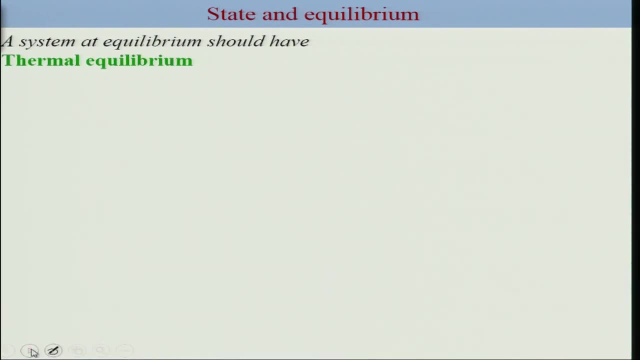 and then you isolate this, this isolate, then there will be no further change in the system because there will be no interaction with the surrounding. So that is how we are going to define the equilibrium. So in many form of equilibrium a system is said to be at equilibrium when all kind 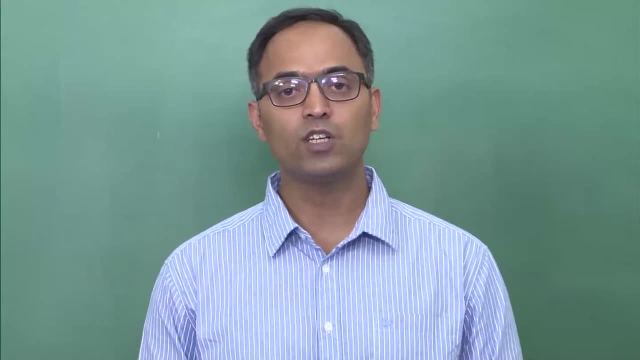 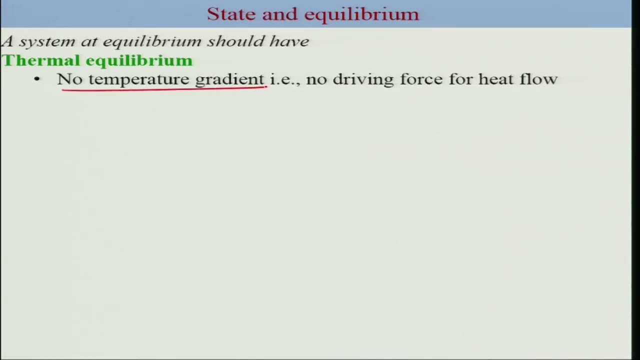 of equilibrium conditions are met. The equilibrium conditions are thermal equilibrium, mechanical equilibrium, chemical equilibrium. So let us look at one step by step. Thermal equilibrium will be where there is no temperature gradient, that means there is no driving force for heat to flow. A mechanical equilibrium is when there is no change in the pressure with time. 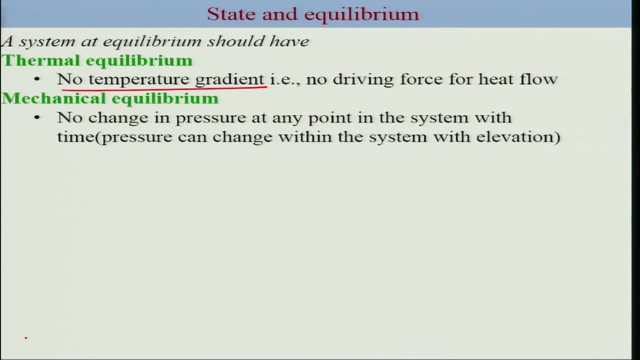 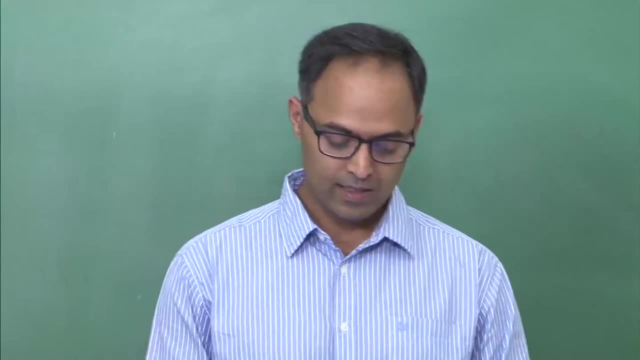 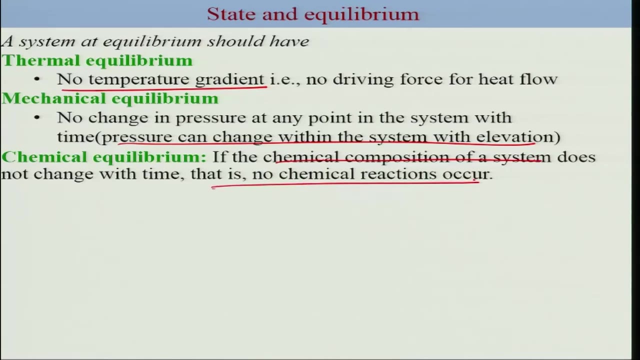 So there is no driving force for a fluid to flow. So pressure can change within the system with elevation, but in such case the forces will be balanced. Then you have this chemical equilibrium. So if there is no changes in the chemical composition of a system, then the system is at chemical equilibrium. So 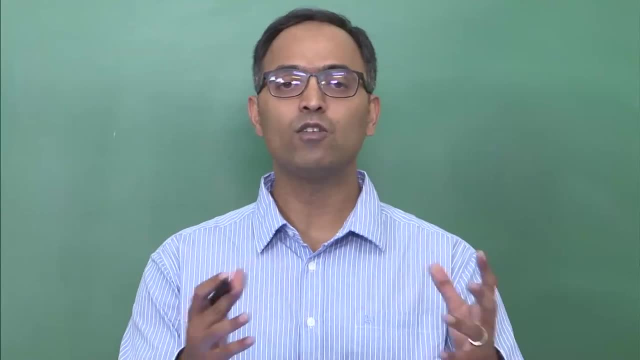 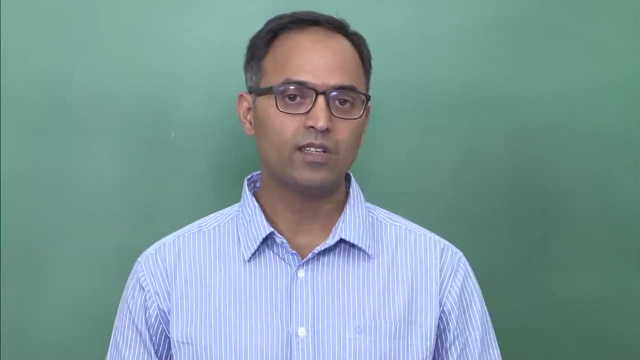 for example, you can consider like sugar dissolved in water and there is no changes in the chemical composition throughout the your system and it will be said at chemical equilibrium. Now there is something called phase equilibrium. Now, this is relevant when you have more than. 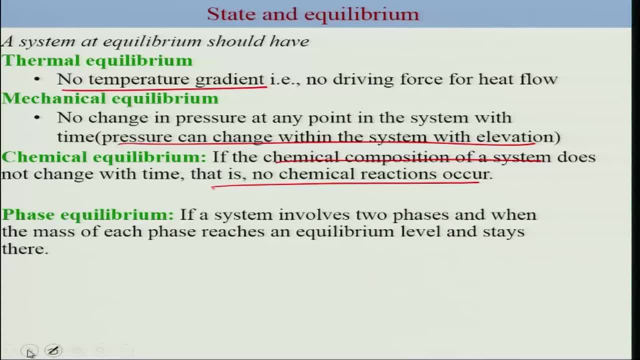 one phases, So phases such as liquid, gas, solid. So if you have, for example, the two liquids, let say oil and water, after you shake and you let it to stay for a while, the oil separates and the water separates and there is no change. in the composition of the oil and as well as in the composition of the material. Then all these tried complex木 is destroyed. But whatever happens, if the liquid divines some way, the material does not, turning to solid fluid every 5 days. So when you have such 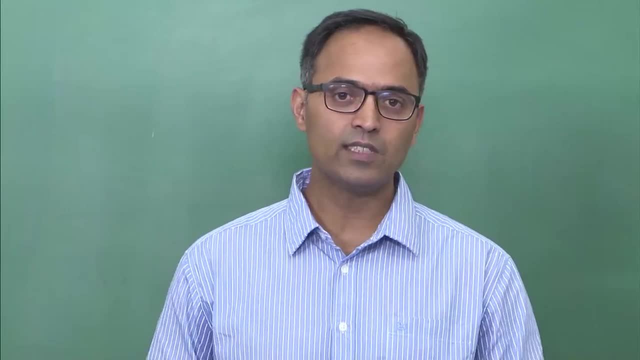 a state, then why to think is said to be solid fluid. Let us work to measure this. If you water after a while and they will be considered to be at equilibrium because they will meet the thermal equilibrium. they will meet the phase mechanical equilibrium as well as they 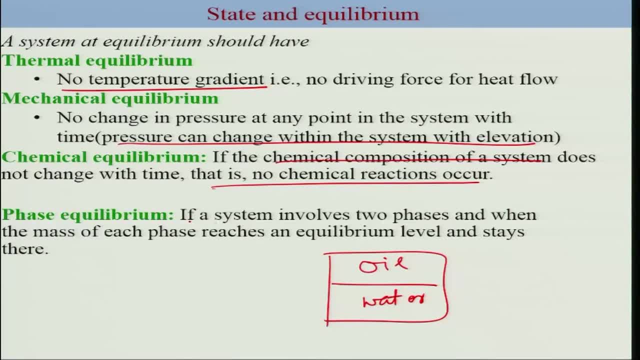 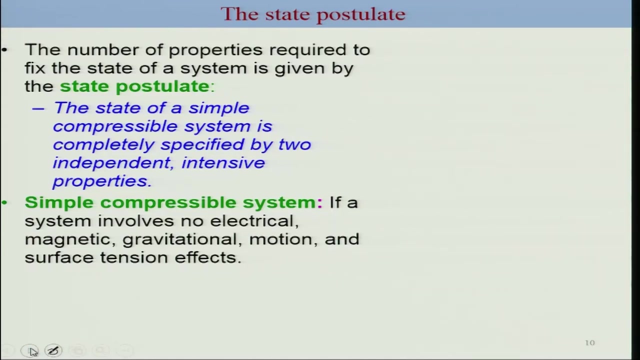 are at phase, two different phases, So hence a phase equilibrium is a system which involves two phases, and when the mass of each phase reaches an equilibrium level, they and stays there. So this is an example of phase equilibrium. all right, So now we know that the state has a series of the properties, or set of properties, and 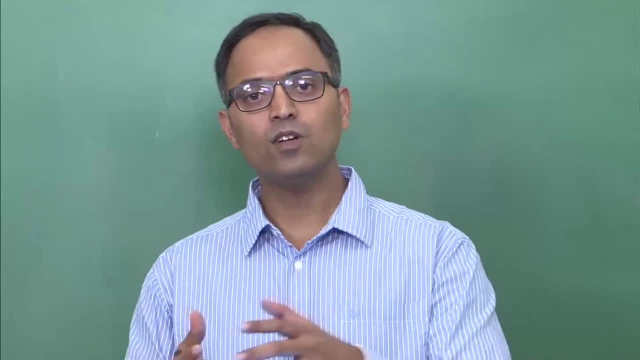 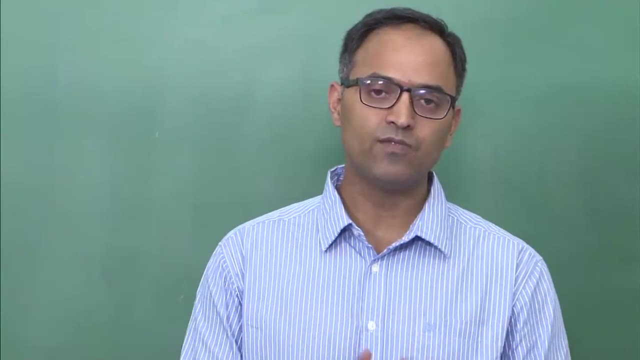 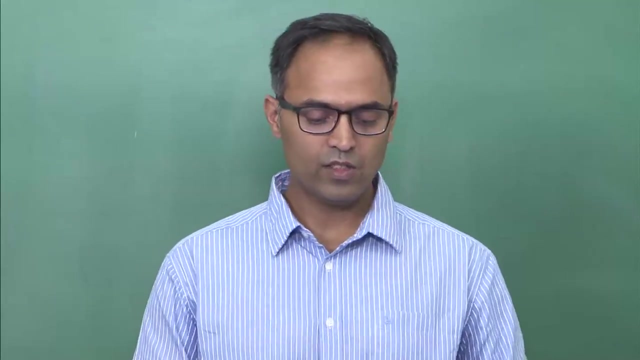 if you change one of the property, the state will change. But it is not necessary that you have to define all the property to fix a state. there is a minimum number of properties which you must define. the rest of the property gets fixed upon once you define this minimum number and that is how we the state. that is what the 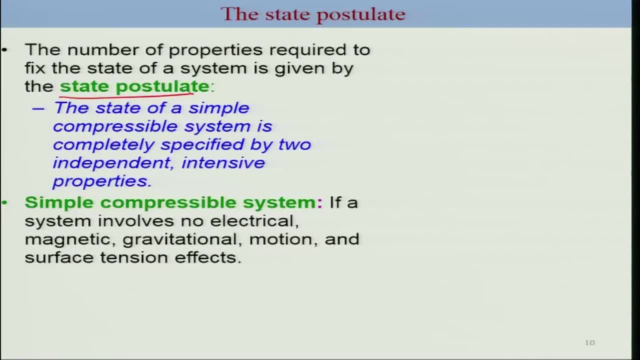 state postulates tells us. So state postulate is the state of a simple compressible system which is completely specified by two independent intensive properties. ok, Now what is a simple compressible system which is a system which involves no electrical, magnetic, gravitational and surface tension kind of component? 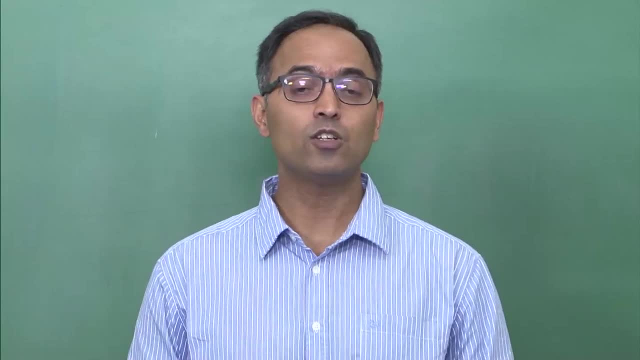 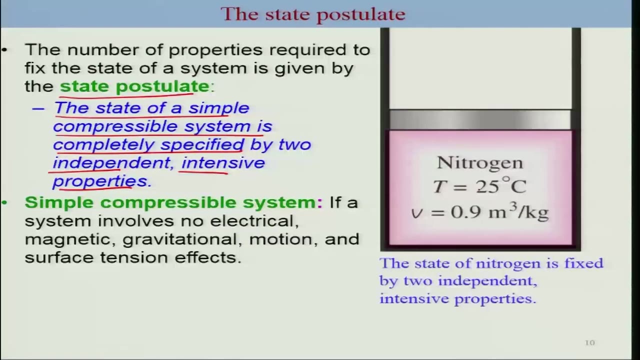 If you have those, then you have to include another variable in order to define the state. Now, this is an example of a specific state where So just two variable has been defined: temperature and specific volume. ok, Now you can. you can make use of temperature and pressure also, but this is relevant only. 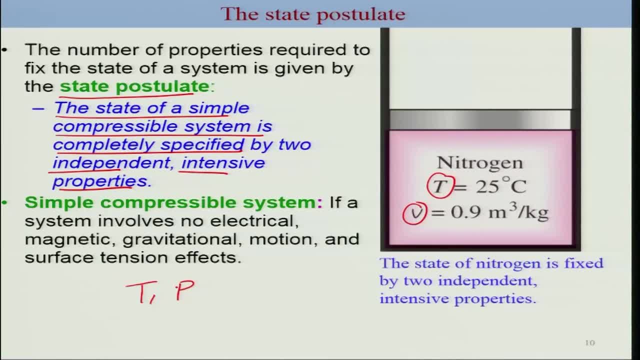 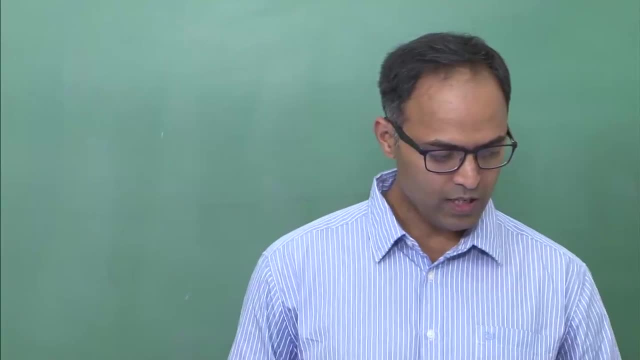 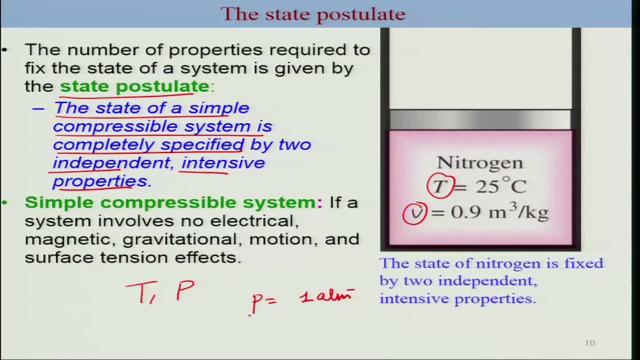 for single phase. for single phase temperature and pressure are independent. but for two phases, for example where water liquid is converted to vapor, then the temperature pressure gets related. So this is a kind of an example Where you know that at sea level, when the pressure is one atmosphere, water boils at. 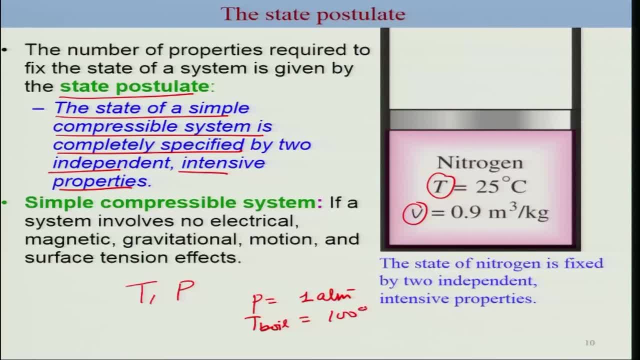 100 degree Celsius right. and when you go to the mountain the pressure is less than atmospheric pressure and the boiling temperature also gets reduced and in such cases when there is a phase change. So temperature is a function of pressure, the temperature of the boiling temperature. 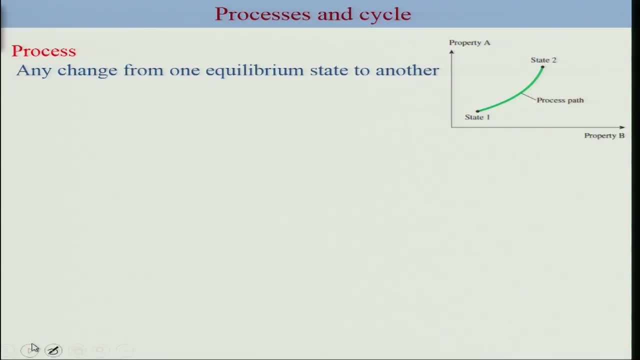 is a function of pressure, Any state you can change along during the process. so we will be defining the process here, that any change from one equilibrium state to another. So this is an equilibrium state and this is an equilibrium state and this is a process. 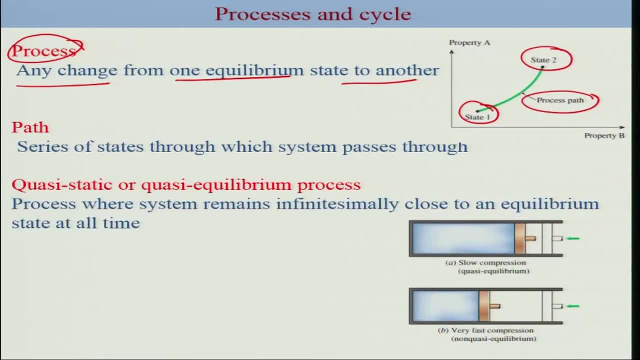 path. ok, So a process path is the series of state through which the system passes through. So essentially, it means that each of them along this green line, This is the state and this is the specific state. this is the specific state of our interest. 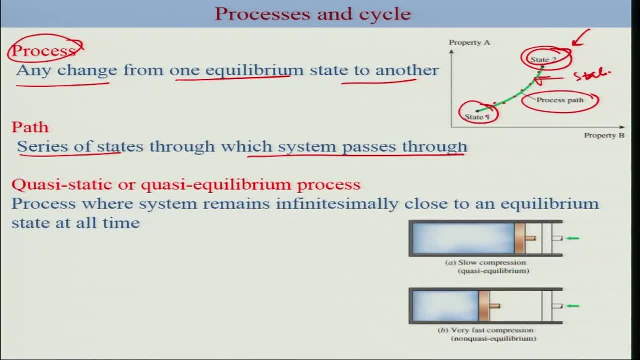 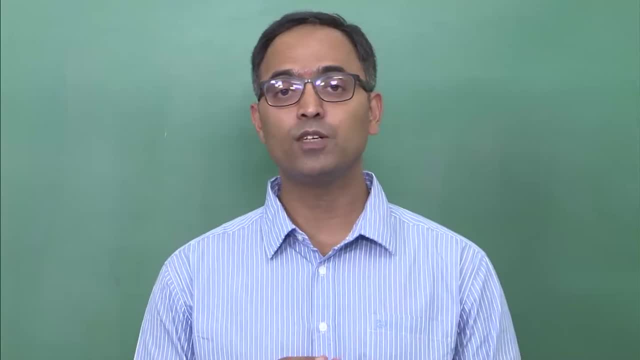 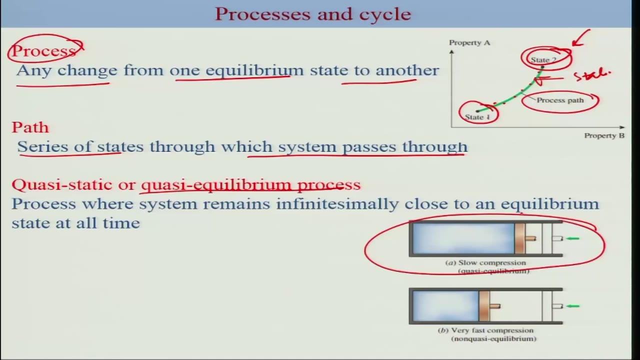 So there is a process which are very fast. there is a process which are very, very slow. a slow process where the intermediate point along the path are at equilibrium, or quasi equilibrium is called quasi equilibrium process. So this is an example. there you are using the slow compression in order to reach in.